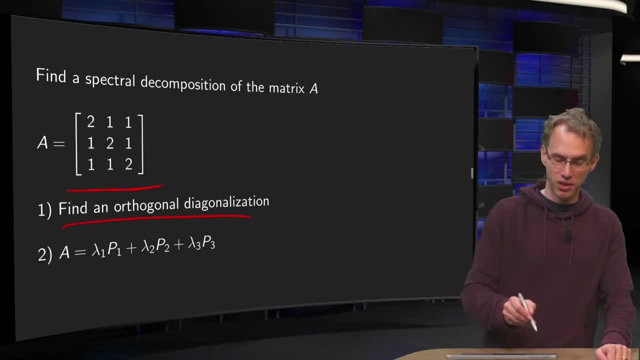 That is the first step, And once we have that, we can rewrite our A as λ1- p1 plus λ2, p2 and λ3- p3. So then we have to find the p1, p2 and p3. Well, most work is actually to find an orthogonal diagonalization. 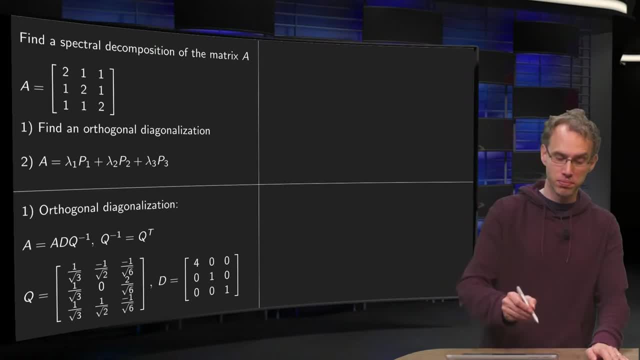 We have done so in earlier examples, so I will just give the result here. A equals should be q times z times q inverse, where q inverse equals q transpose, And in this case we have eigenvalues for 1 and 1.. So there you have your d. 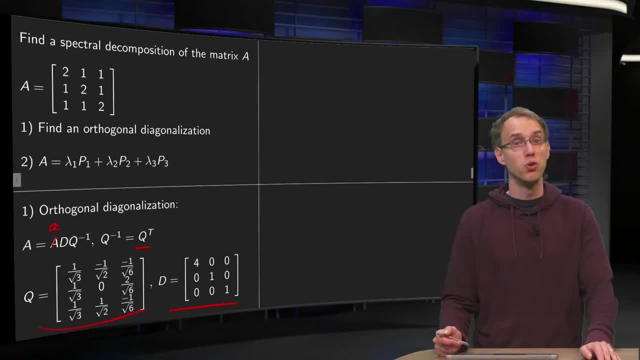 Your q looks a bit ugly, but that is because you have to normalize all columns. orthogonal matrix has orthonormal columns, so there are orthogonal and f-length ones, So those q's usually look a bit ugly. So once you have found this orthogonal diagonalization, it is quite straightforward to make the spectral. 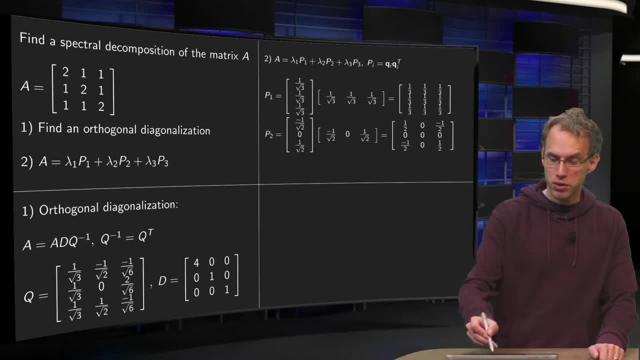 decomposition. So what you have to do is compute the p1, p2 and p3 with pi equals qi times qi transpose. So there you have your d. Your q looks a bit ugly, but that is because you have to normalize all columns. 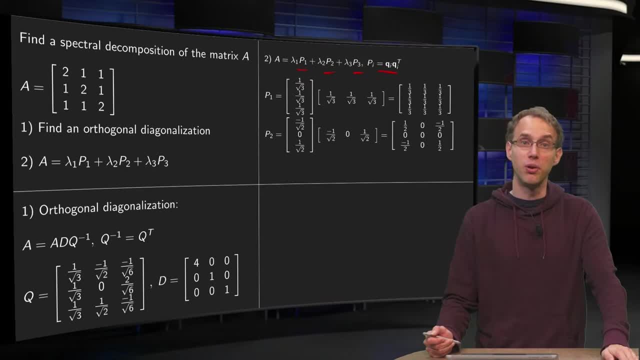 So here you have your p1 equals q1 times q1. transpose. Now you have q1, q2 and q3 already Those are the columns of your matrix q. So your p1 equals q1 times q1. transpose. You can use, for example, row column rule: 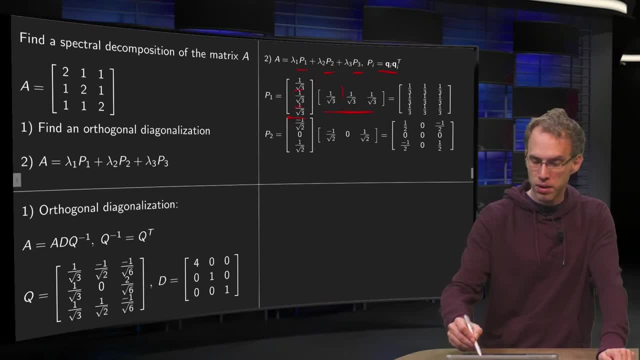 Here we have a bunch of rows and here a bunch of columns. So 1 over square root of 3 times 1 over square root of 3 yields 1 over 3. Also for all the other elements. So it gives you your first column of the product. 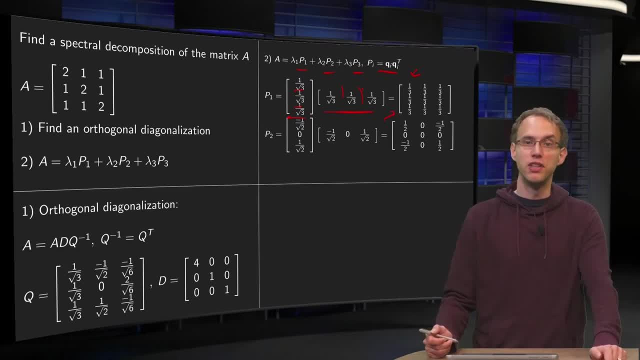 And that is 1 over square root of 3.. And the second and third column is completely symmetric, so they are the same. So there you have your matrix, P1.. And then for P2, the same row-column rule again. So here a bunch of rows, here a bunch of columns. 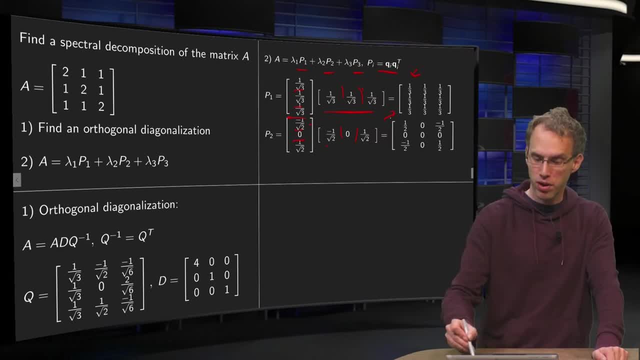 So minus 1 over the square root of 2 times minus 1 over the square root of 2 gives you 1 half. Zero times minus 1 over the square root of 2 gives you a zero One over the square root of 2 times minus 1 over the square root of 2, minus 1 half.